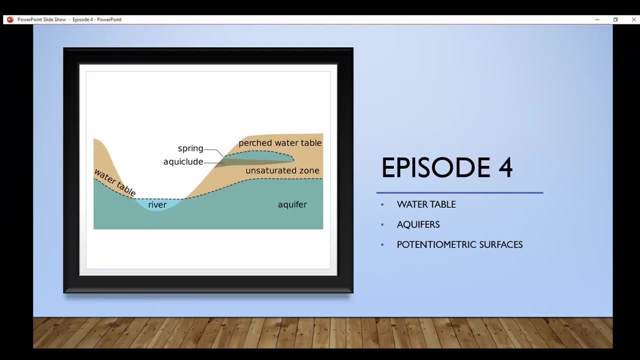 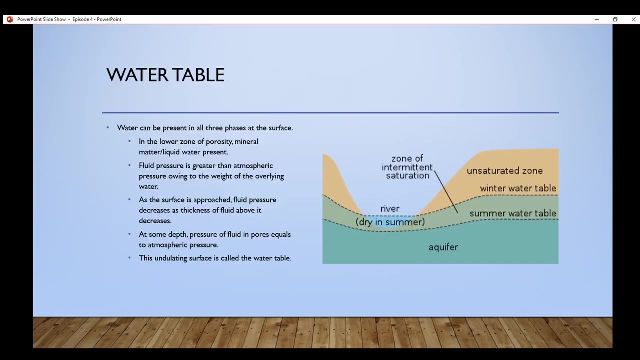 What's going on everybody? Welcome back to the Hydrogeology playlist. This is episode 4 and in this episode we'll be covering water table, aquifers and poniometric surfaces- A lot of important concepts in this episode. So the water table? Okay, water can be present in all three phases at the surface, which can mean solid as ice, gas, as water vapor and as liquid running water or precipitation rain. 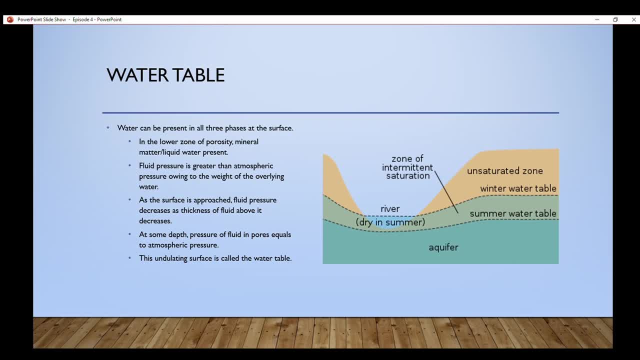 In the lower zone of porosity, mineral matter and liquid water are present, which means basically at the bottom of an aquifer. when you start getting deeper into the crust, Fluid pressure is greater than the atmosphere Atmospheric pressure. owing to the weight of the overlying water and as the surface is approached, fluid pressure decreases as the thickness of the fluid above it decreases. 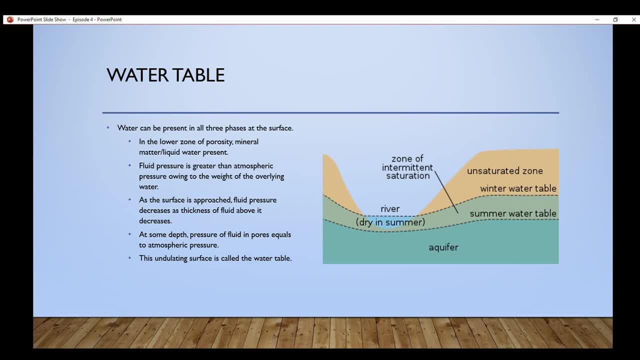 And at some depth, pressure of the fluid in the pores of an aquifer, for instance, equals to the atmospheric pressure, And this surface is called the water table. this undulating surface And atmospheric pressure and porosity pressure Or fluid pressure are equal at these lines is basically what that says. 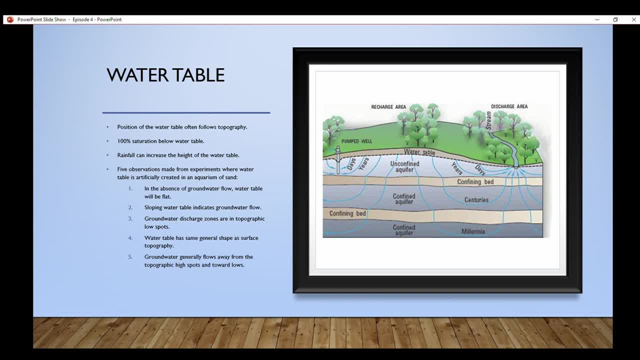 So the position of the water table often follows topography, with hills or valleys, And there's 100% saturation within the rock below the water table or within that geologic material. Rainfall can increase the height of the water table or decrease, like this one shows. 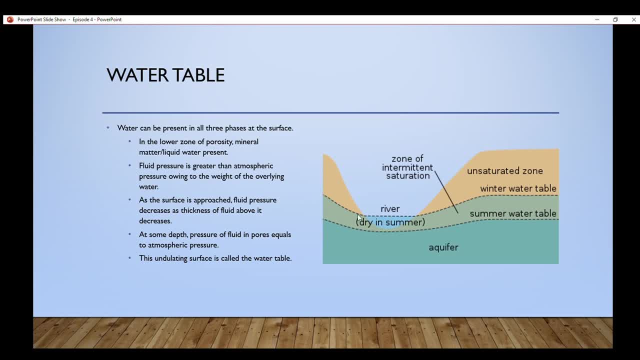 You have the summer water table Because rain is less, it's drier in the summer, like it says right here, And then in winter, if you have a lot of snow, melt it can increase And if you have a lot of precipitation it can increase the height of the water table. 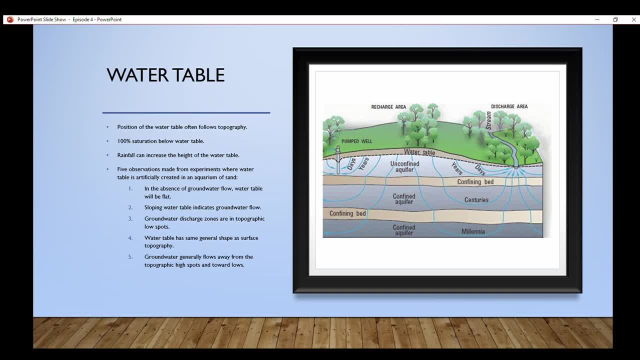 And five observations have been made from experiments where water table is artificially created in an aquarium of sand. They basically use a spray bottle and spray the sand, Kind of signifying rain precipitation, And over time that builds up an actual water table in the aquarium. 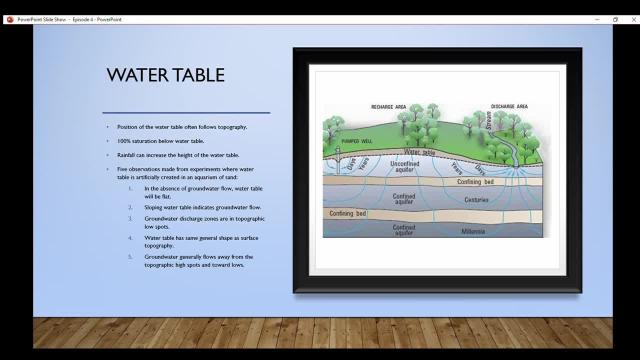 Kind of cool. I think that's going to be my son's science project. So in the absence of groundwater flow, a water table will be flat And then a sloping water table indicates groundwater flow. Groundwater discharge zones are in topography. 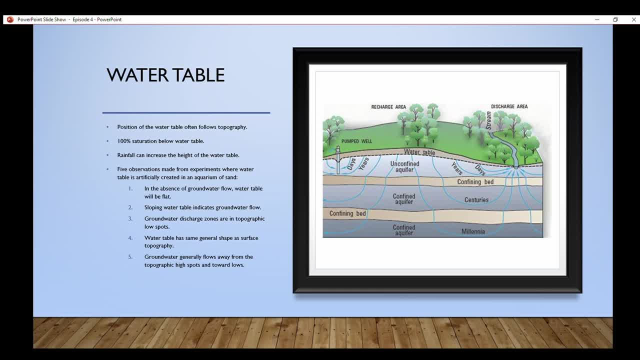 Topographic low spots, so, like in a valley where there's a stream Water table, has the same general shape as the surface topography. as you can see in this picture, You've got a little hill, so the water table is higher at this point than it is in the valley, in the stream valley. 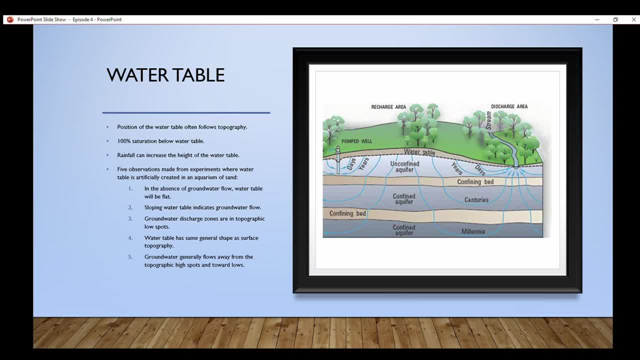 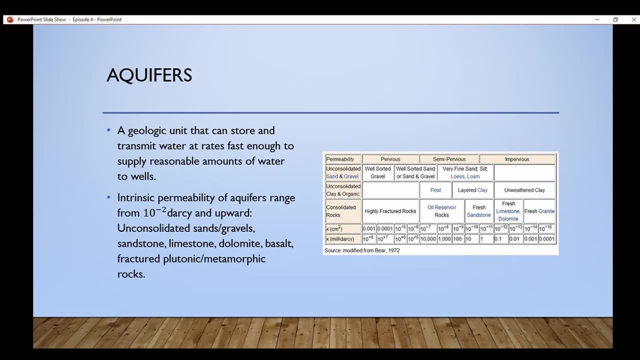 And then groundwater generally flows away from the topographic high spots and towards the low spots. A geologic, okay. so an aquifer is a geologic unit that can store and transmit water- Water at rates fast enough to supply reasonable amounts of water to wells. 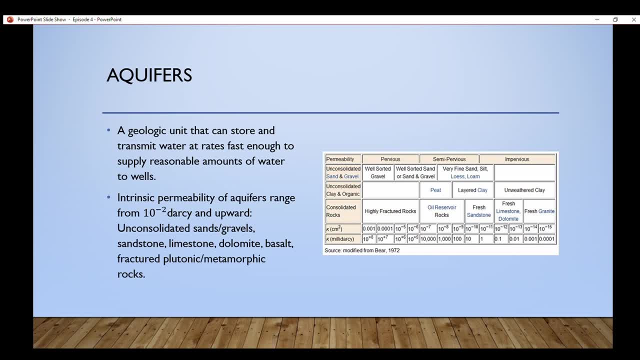 And your intrinsic permeability of aquifers ranges from 10 to the negative second Darcy and upward. So you've got unconsolidated sands, gravels, sandstone, limestone, dolomite, basalt, fractured plutonic and metamorphic rocks. 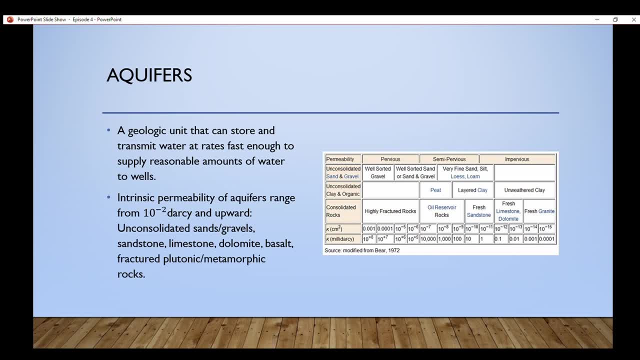 Just like we talked about during that porosity episode. Typically plutonic and metamorphic rocks won't have porosity. They'll pretty much be retardant to water. But if you have it highly fractured, that increases the ability of water to not only seep into that rock but to transmit itself throughout the rock. 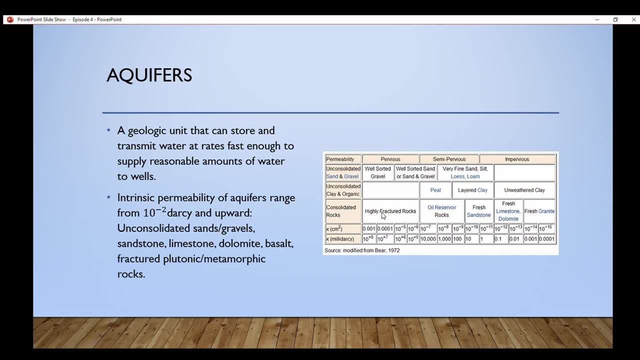 And this is about the point that this is talking about, in terms of intrinsic permeability, 10 to the positive, 5 milliDarcy's, That's 10, yeah, And that converts to about 10 to the negative 6.. 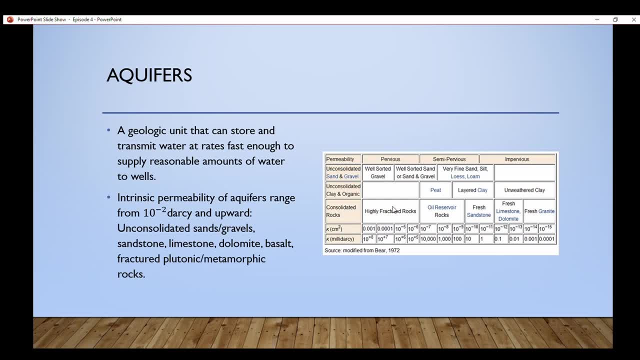 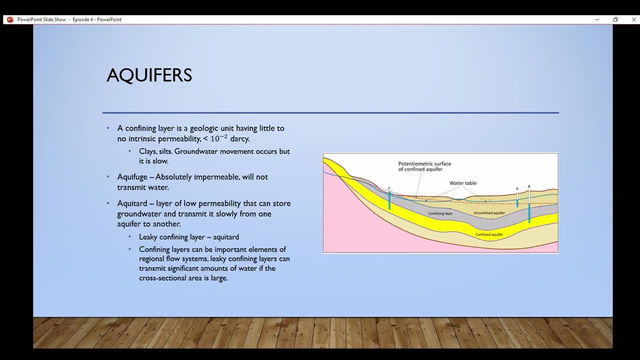 So they're talking basically about in this area in terms of what a good aquifer would be. So a confining layer is a geologic unit having little to no intrinsic permeability, Less than 10 to the negative. 2 Darcy. 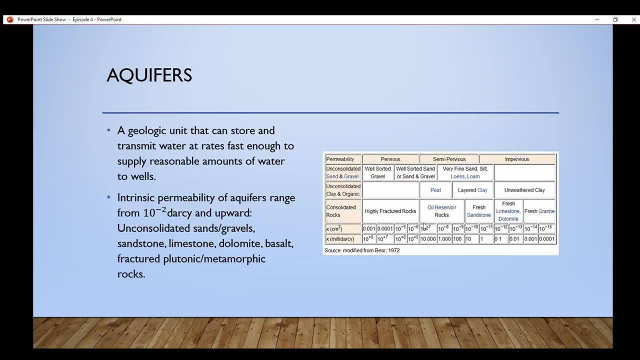 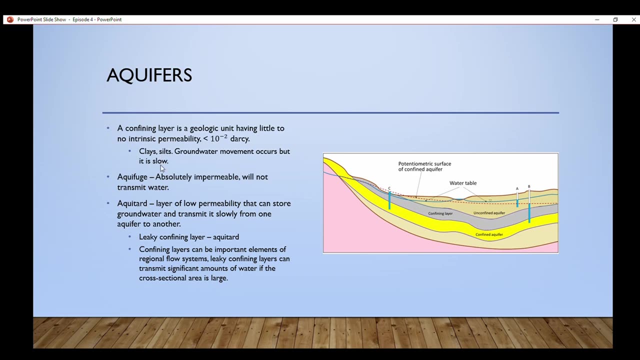 Which is pretty much from this point on. So all these can be confining layers, These particular rocks or sediments. So clay is silts. Groundwater movement still occurs, But it is very slow An aquifuge, And these are a couple different definitions that you'll see when studying hydrogeology. 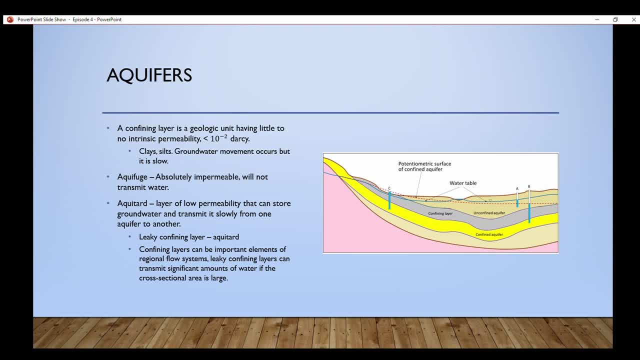 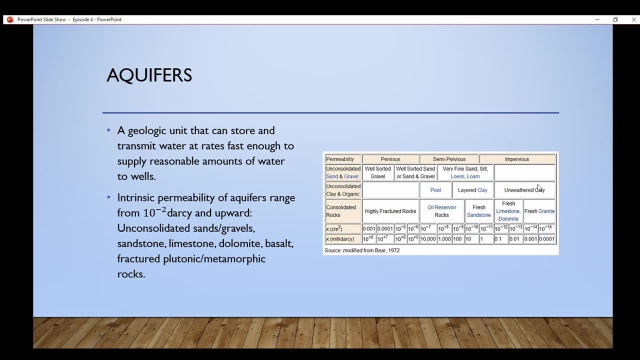 But aquifuge is absolutely impermeable And will not transmit water. Best example of that would probably be a fresh granite Or an unweathered clay In terms of an aquifuge, And an aquitard is a layer of low permeability. 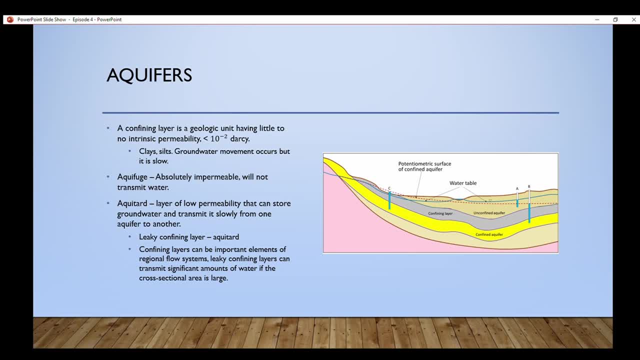 That can store groundwater and transmit it slowly from one aquifer to another, So like a shell, Claystone, siltstone, something like that- And then a leaky confining layer is also considered an aquitard And basically that just means that it's kind of fractured. 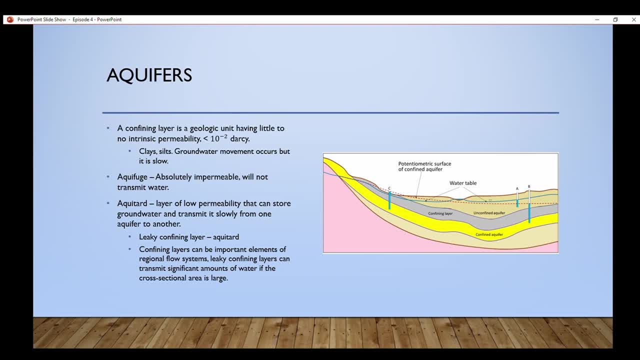 So it's allowing water to transmit through it And eventually reach to the aquifer Through that confining layer, And confining layers can be important elements of regional flow systems. Leaky confining layers can transmit significant amounts of water If the cross sectional area is large enough. 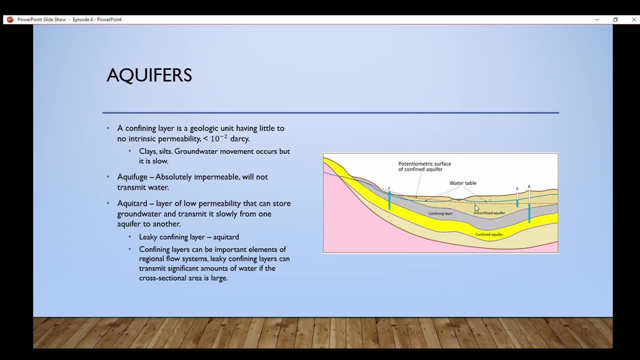 And in this picture you see an unconfined aquifer, Which we'll be explaining what that is- A confining layer And the confined aquifer- And we'll explain a little bit more About the poniometric surface, Which at this point is above the topographic surface. 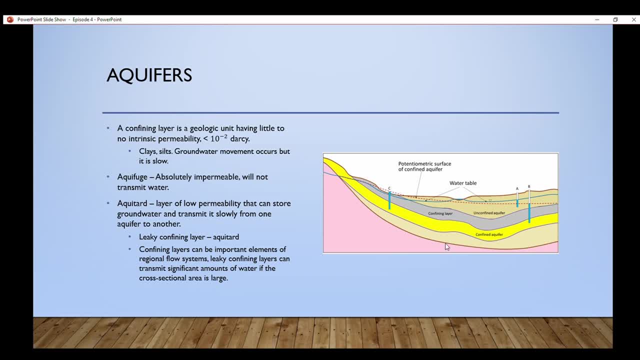 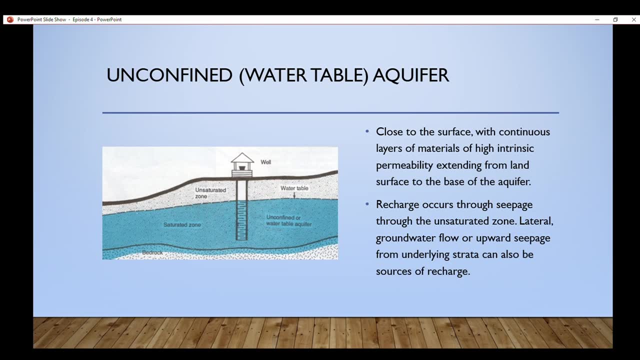 Right here. So an unconfined water table Is also what it's called. Aquifer is closer to the surface, With continuous layers of materials of high intrinsic permeability Extending from the land surface to the base of the aquifer. 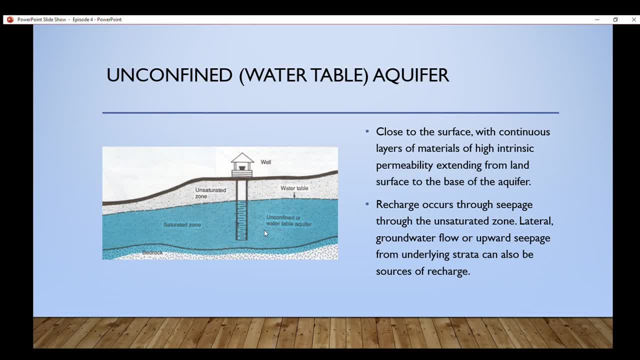 So you know Unconsolidated gravels and sands, Just continuous layers. That would be an unconfined water table aquifer And then recharged to these aquifers Occurs through seepage, Precipitation reaches the surface. 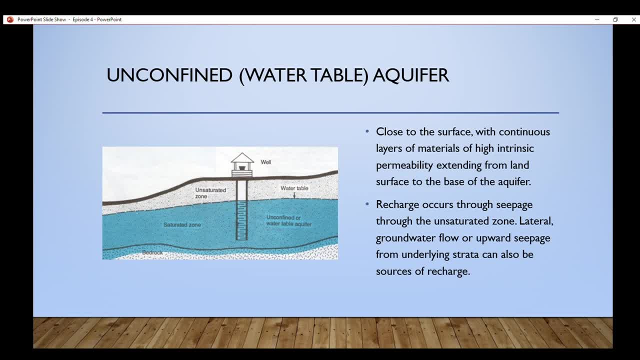 And it starts seeping into the ground. Eventually it reaches the water table And recharges the aquifer. And lateral ground flow or upward seepage From, say, the bedrock. If it has water within it It can escape into the aquifer. 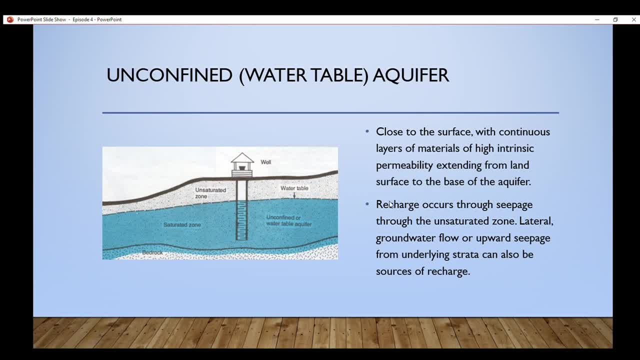 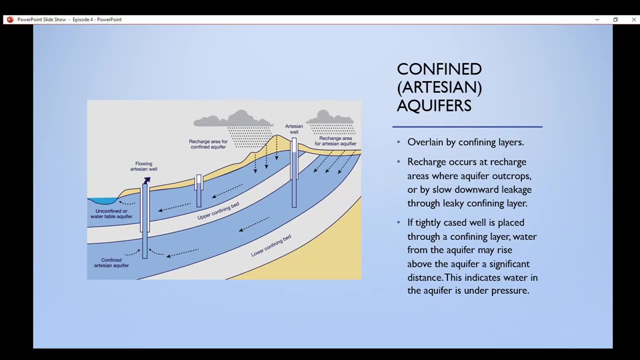 And then lateral ground flow is coming from other sources Say: this is a valley over here With a stream that is losing. That means it's feeding water to the aquifer And a confined or artesian aquifer Is overlying by a confining layer. 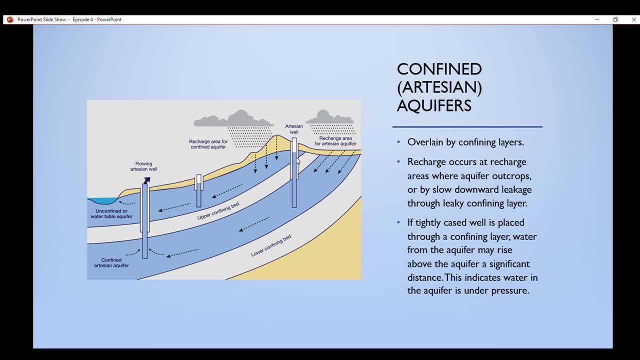 So this is an artesian aquifer, Has a lower and upper confining bed. Recharge occurs at recharge areas Where the aquifer outcrops, So right here, And Or by slowly Slow downward leakage through A leaky confining layer. 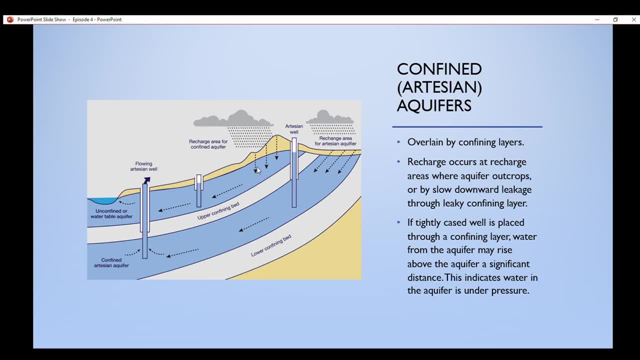 So if rain occurs here, It will eventually reach the confining bed And it can seep through, But at very slow rates. So if a tightly cased well is placed through a confining layer Like this one right here, Water from the aquifer may rise above the aquifer. 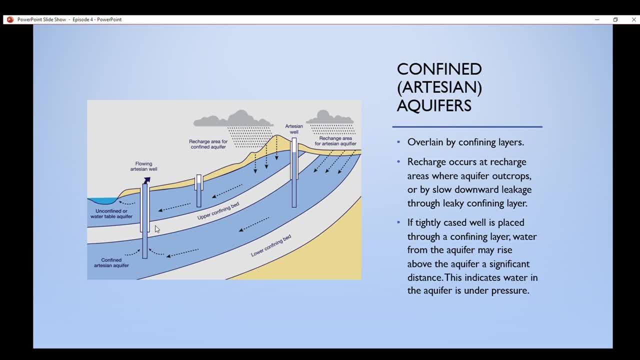 A significant distance. as you can see, The Poniometric surface is right- Well, not the poniometric surface, But the water table of this aquifer is right here. But If you drill a hole into it And release pressure, 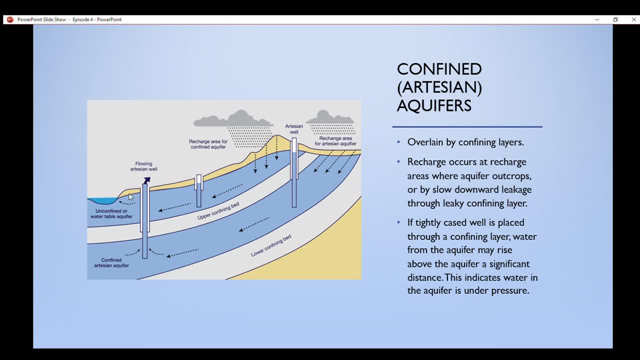 This can become what's called a flowing artesian well, And the water can actually start flowing out of that Because of pressure built inside the aquifer. So it This indicates water in the aquifer is under pressure. Yeah, okay, Poniometric surfaces. 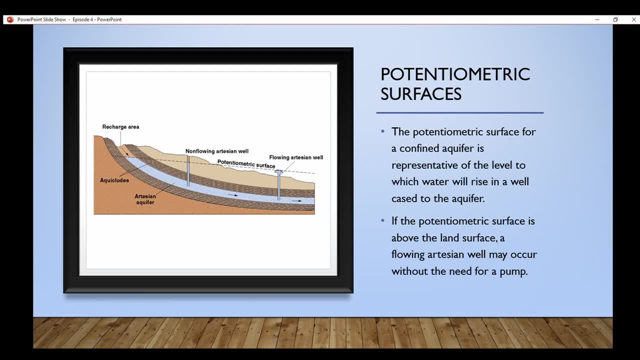 The poniometric surface for a confined layer Is representative of the level To which the water will rise In a well cased to the aquifer, And if the poniometric surface Is above the land surface, like it is here, 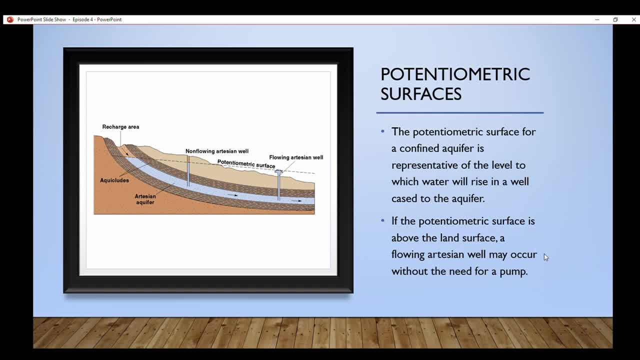 At this point, A flowing artesian well may occur Without the need for a pump. Whoops, And here's a couple aquacludes, As, if you remember, Those are completely impermeable. They don't allow water through them. 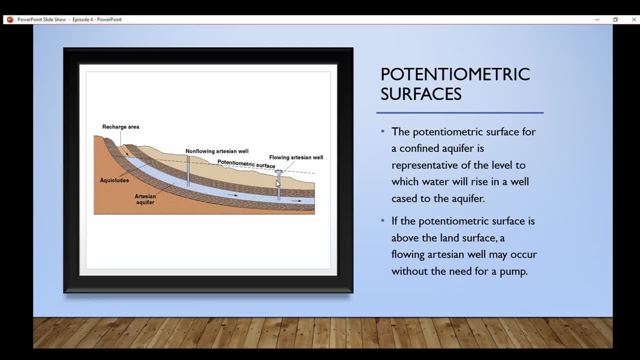 Obviously, a lot of pressure is going to build in that, In that aquifer, And this is the recharge zone Allowing water to Recharge this aquifer. Okay, So, a perched aquifer, And I've dealt with these a little bit. 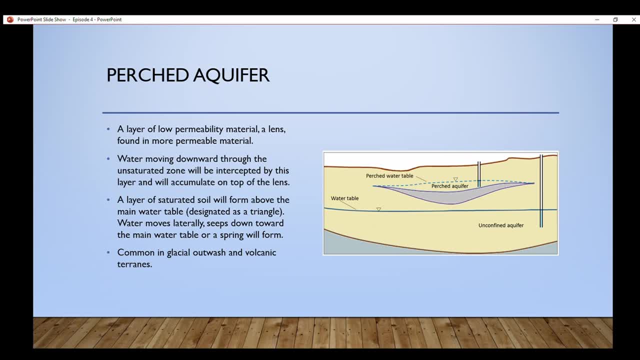 It's kind of cool. A layer of low permeability Material, A lens, As depicted here, Is found in more permeable material, So in some cases, If you have a river, Siltstone or sandstone, You can have interbedded lenses of clays. 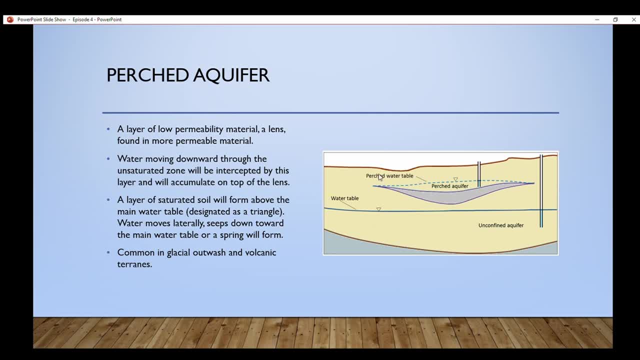 Occur. That's a good example of How a perched aquifer can form. Water moving downward Through the unsaturated zone Will be intercepted by this layer And will accumulate on the top of the lens, So as you can see. 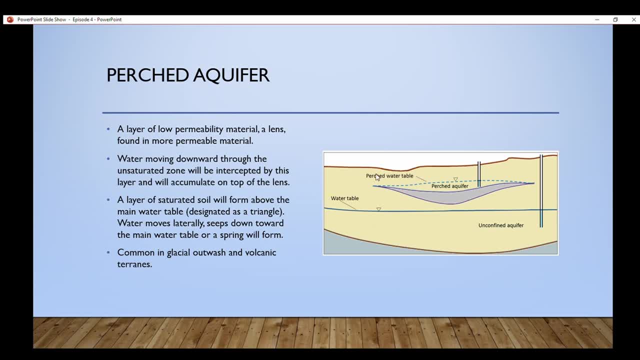 This perched aquifer has it's own water table. A layer of saturated soil Will form above the main water table, Which is A triangle. You'll see this symbol a lot. The triangle basically just signifies Where the water table is. 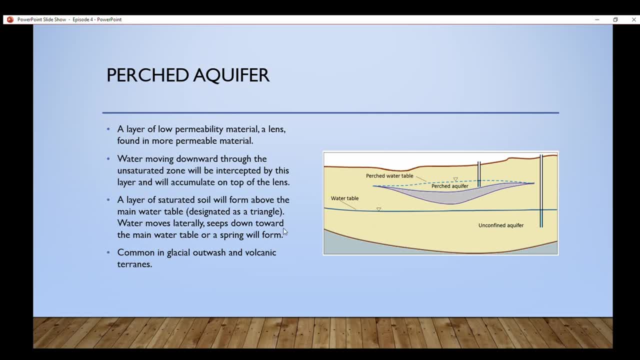 That's a symbol that they'll use. Water moves laterally, Seeps down toward the main water table, So it comes off like this And it will Either seep down to the main water table Or a spring will form, If the topography allows it. 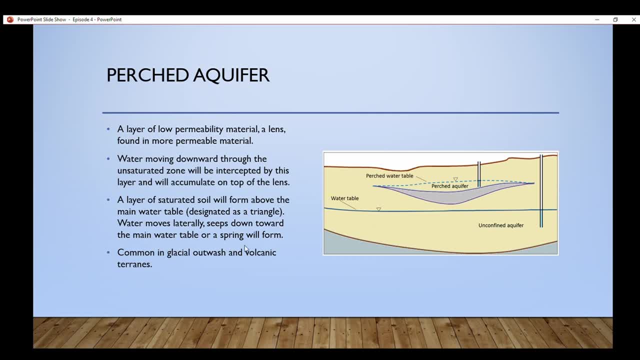 And then It's common in Glacial outwash In organic terrain, So a glacial outwash, As we talked about before. Glacial till Is poorly sorted. You get a lot of different materials: Gravels, Clays. 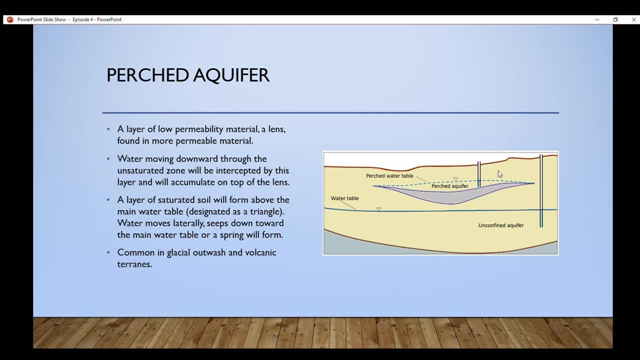 Silts Sands, You get everything in a glacial till And, as you probably can figure out, There would be some certain situations Where you might have more clay Than gravels In a certain area, Which can create a lens. 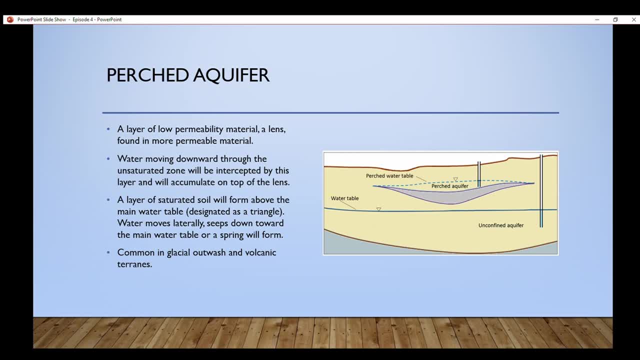 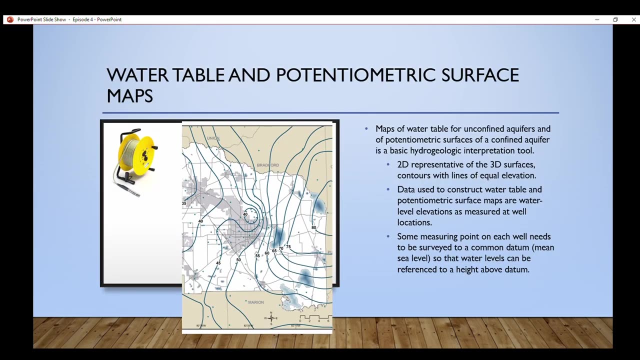 And then in volcanic terrains You can have basically alternating sequences, Like in a cinder cone volcano Of basalt And volcanic ash, And that can create Perched aquifers as well. So a water table And poniometric surface maps. 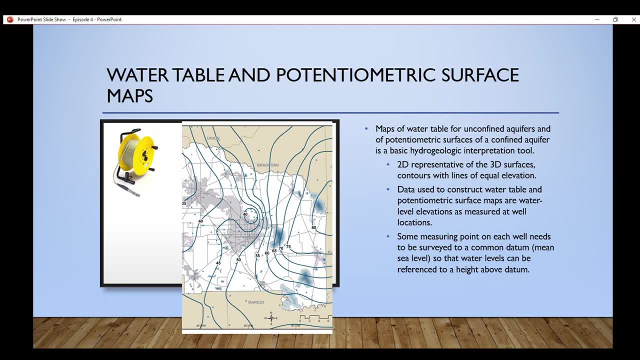 This is actually what I Tend to do Professionally In my job, And I actually use this tool, The water level gauge. This indicates Not only water level, But if there's petroleum product Within the water, The well. 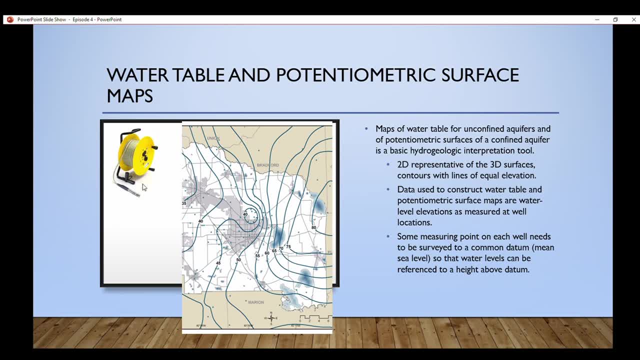 It'll have a solid beep And that'll tell you that there's product Gasoline Oil, Because obviously those are lighter density Than water, So they'll float to the top Typically, But anyways. Maps of water tables For unconfined aquifers. 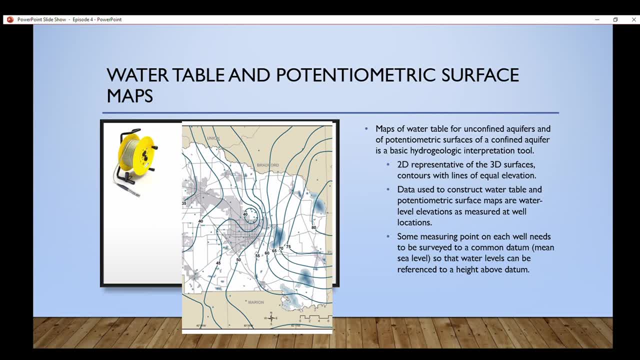 And of poniometric surfaces of a confined aquifer Is a basic hydrogeologic Interpretation tool. You have a 2D representative, Which is this map right here Of the 3D surface contours With lines of equal elevation. 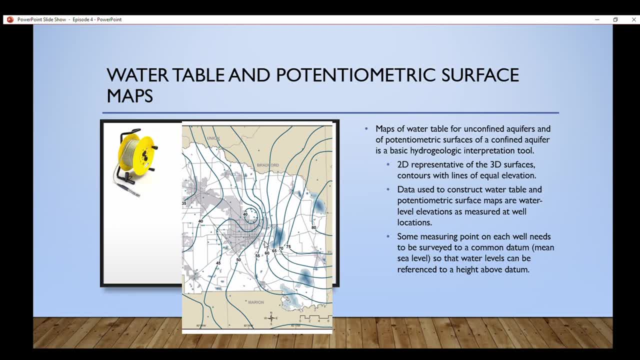 That's what each of these lines indicates. You have a Ground water elevation Of 60 at this particular line, And Data used to construct these water tables And poniometric surface maps Are water level elevations As measured at well locations. 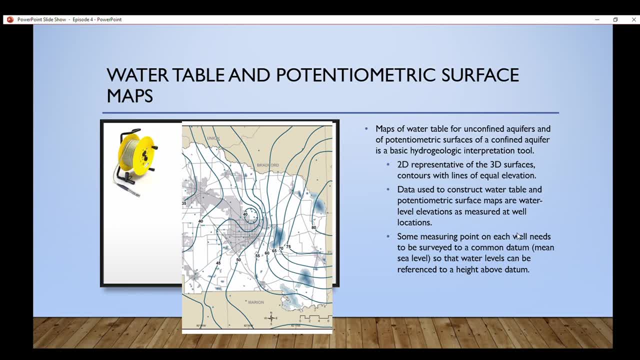 Using this Or some other type of device And some measuring points On each well needs to be surveyed To a current Common datum Which can mean sea level, So that the water levels can be referenced To a height above datum. 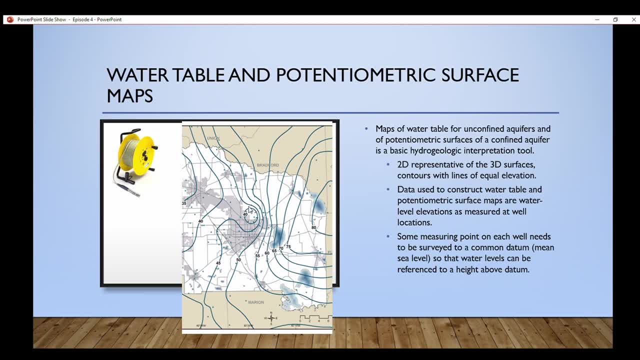 And to add on to this, We also survey If a sea pipe in a well Might be higher at some point. So you have to account for that When you're determining water level. That's something you have to account Into your calculations. 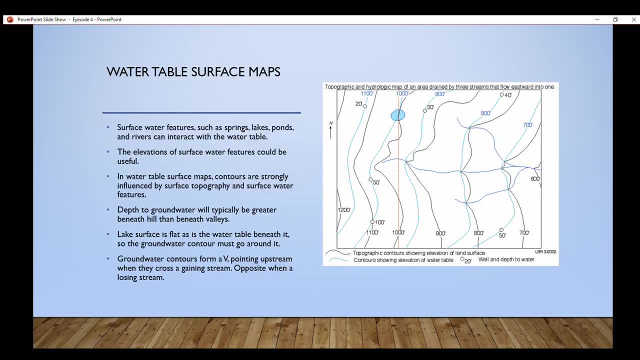 And the elevation point At that particular. well, So in particular Water table surface maps, Which in the professional world We just call them all Poniometric surface maps, But in the book They kind of designate Water table and poniometric. 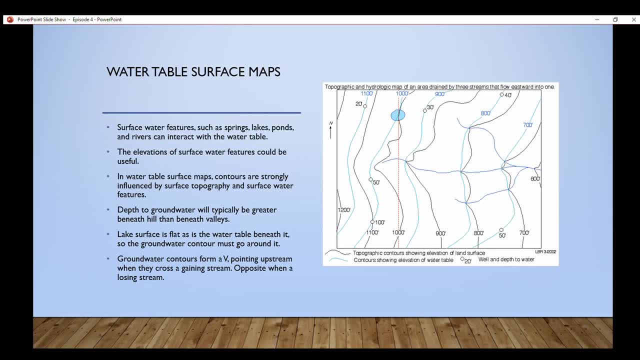 Because water table signifies Unconfined aquifer, So a surface water feature Such as a spring, A lake, A pond Or a river Can interact with the water table. These elevations of surface water features Could be useful. 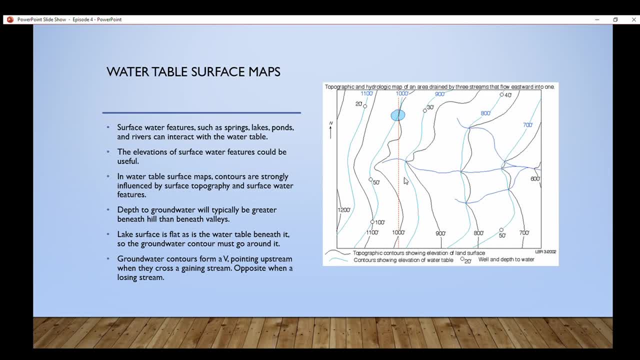 Such as this lake. right here There's a couple streams, Three streams. Knowing the elevations of those Are strongly influenced By the surface topography And surface water features. Depth to ground. On this map, The black lines Are topographic contours. 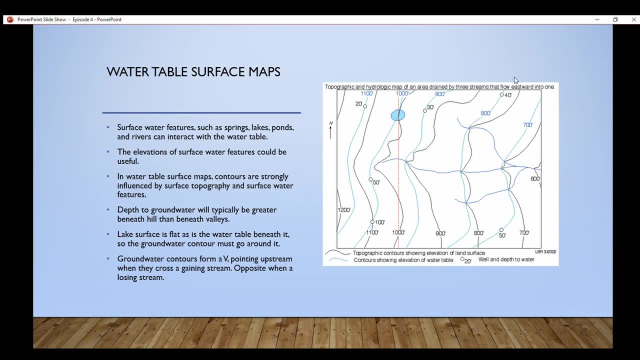 And, as you can see, They for the most part Kind of mimic each other. There's some pattern differences, But they mimic each other For the most part. So where was I? Beneath valleys? So, as we explained a little bit earlier, 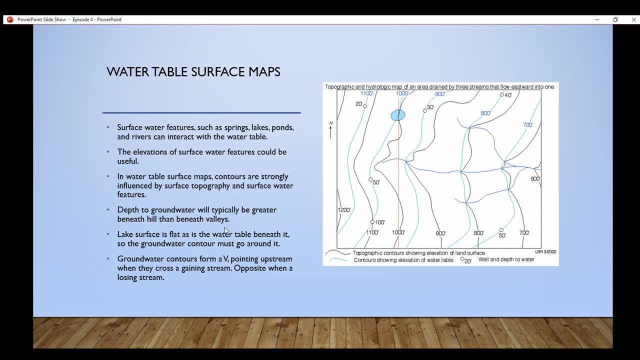 Lake surface is flat, As is the water table beneath it. So here's a lake. The water table And the lake Will have the same Ground, water contour, really Same elevation, But on a water table surface map It goes around the lake. 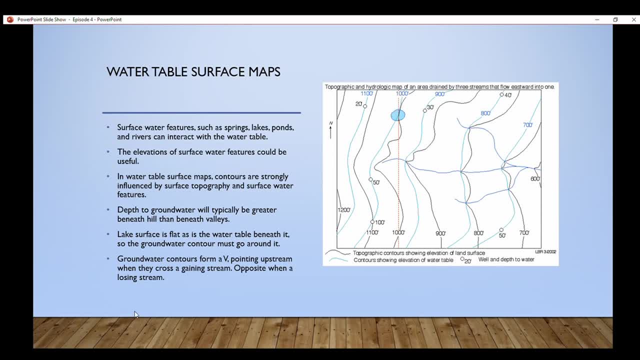 So that's actually a mistake on this map. According to the book, Ground water contours form a V. So you can see some V's Formed on these streams And they're actually pointing in the opposite direction, Which means they are a losing stream. 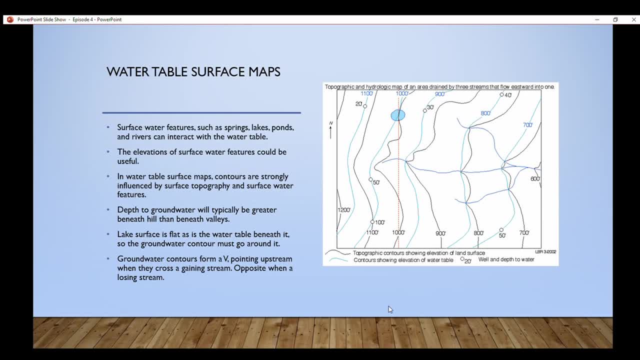 But if they're pointing towards, You know, up the stream, Then, Oh wait, no, These are actually gaining streams. I had to think about it. And if these are pointing In the opposite direction, Then that means they're a losing stream. 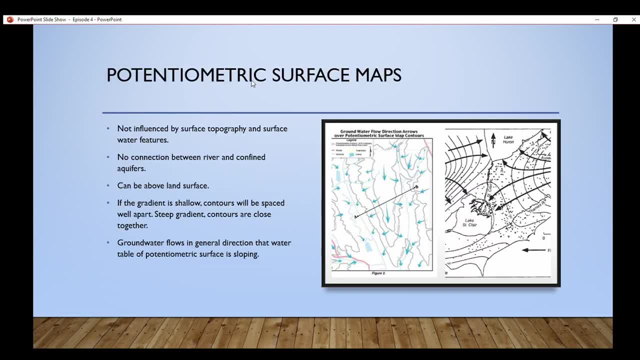 Okay, So poniometric surface maps. They aren't influenced By surface Topography And surface water features. There's no connection between river And confined aquifers And if you think about it from a cross sectional standpoint, That makes sense. 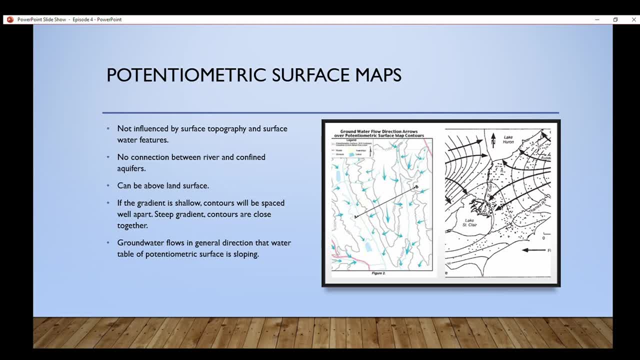 Unless the confined layer is leaky And Poniometric surface elevations Can be above the land surface, As we explained. When it comes to a flowing artesian well, If the gradient is shallow, Contours will be spaced well apart.